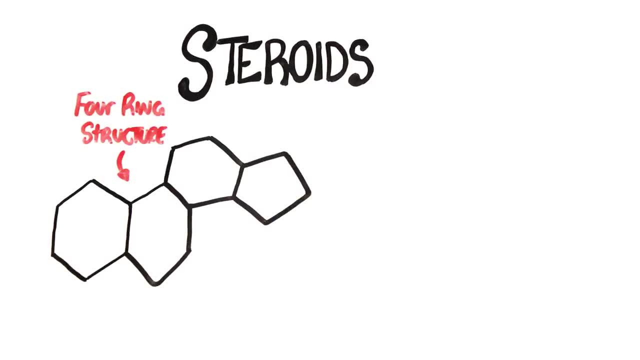 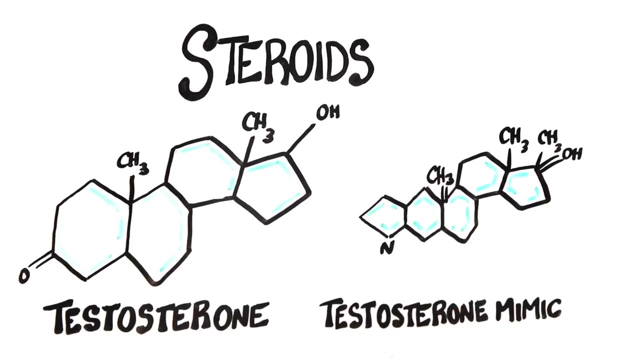 Now, steroids are any compound with a specific four-carbon ring structure, so the term steroid actually includes some chemicals that can be used to treat fever and headaches, and even sex hormones like estrogen and testosterone. But the type of steroid we'll be looking at actually mimic natural testosterone with the intention to enhance performance. 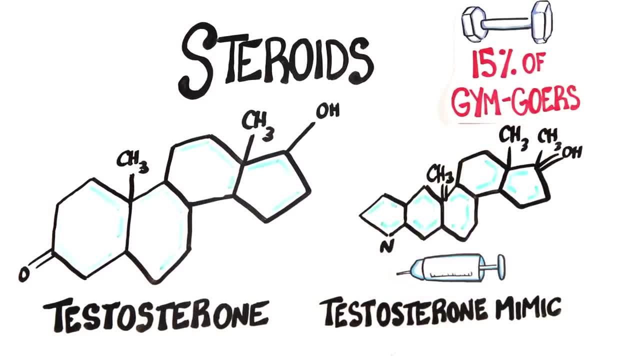 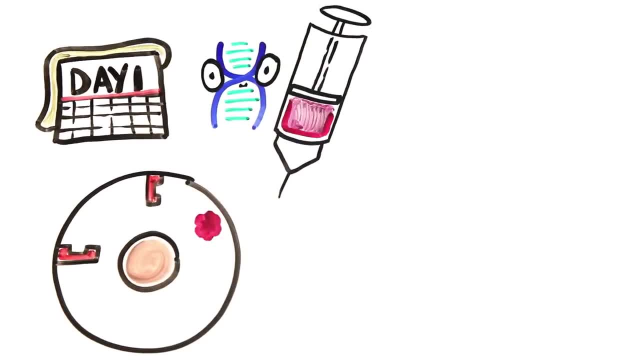 and are used by more than 15% of gym-goers. Within a single day of taking steroids, the expression of your genes will begin to change. Steroids easily enter your cells and bind to the androgen receptor. At this point they can move into the nucleus and attach to your DNA. 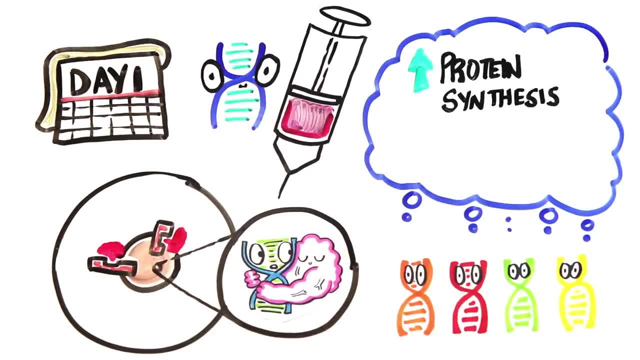 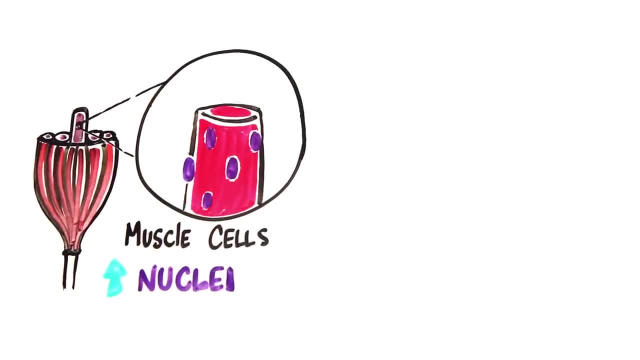 which activates hundreds of genes to increase protein synthesis while slowing protein breakdown. In the end, people who take steroids can have three to five times more nuclei in some muscle cells. Steroids can also stop the differentiation of fat stem cells and decrease a person's body fat. 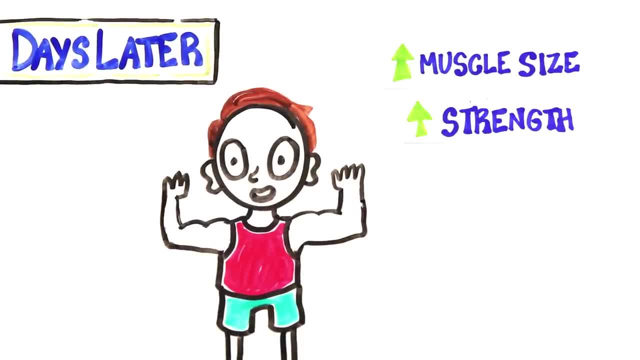 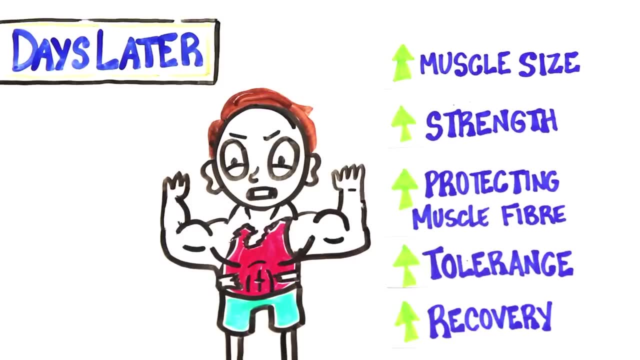 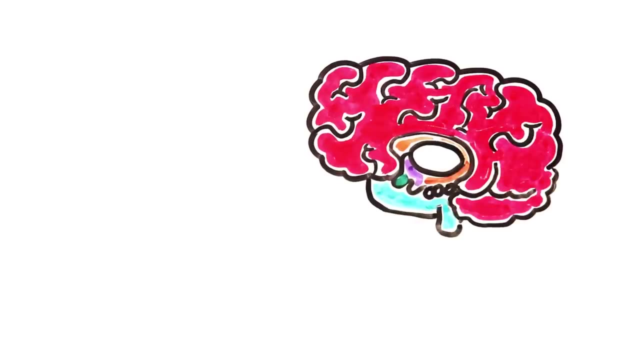 Days in and you're quickly increasing muscle size and strength while also protecting muscle fibers against damage, making steroids ideal for exercise tolerance and recovery as well. But continue to take them and your behavior may start to change, Because steroid receptors are found in parts of our central nervous system. 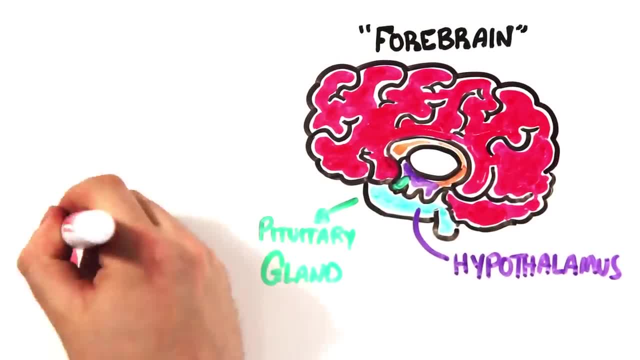 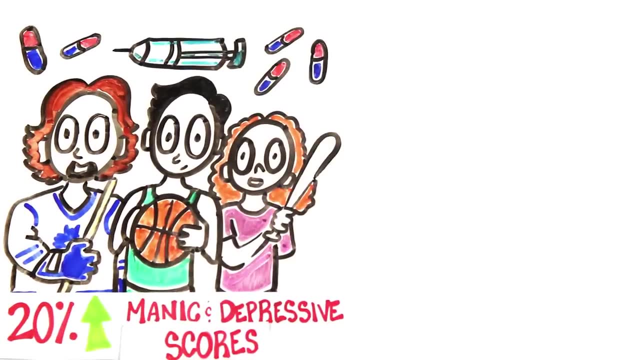 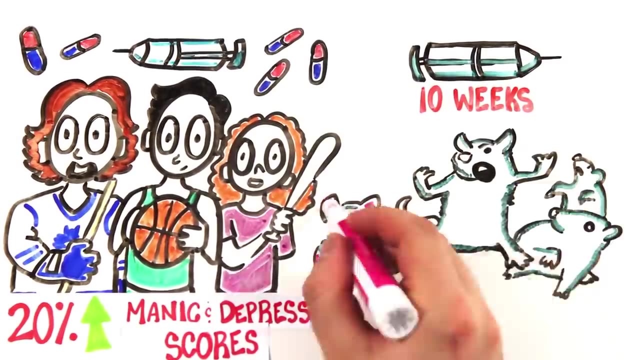 like the forebrain, hypothalamus and pituitary gland, steroids can lead to the classic ROID RAGE. A study of athletes taking steroids showed 20% developed higher manic and depressive scores than non-users. Mice given steroids over 10 weeks also become more aggressive towards other mice put in the same cages. 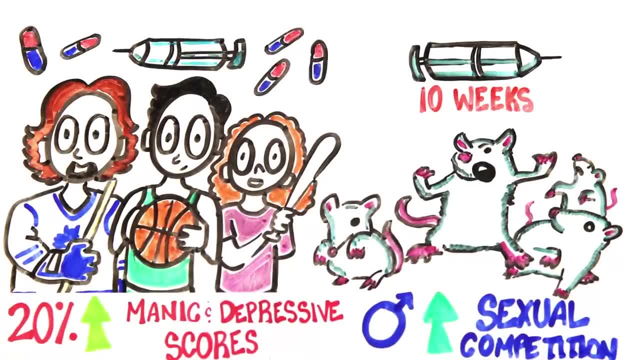 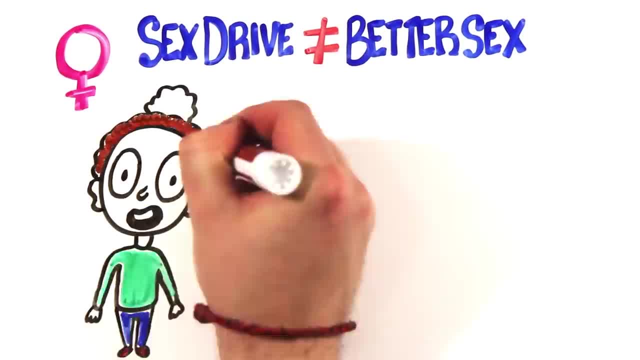 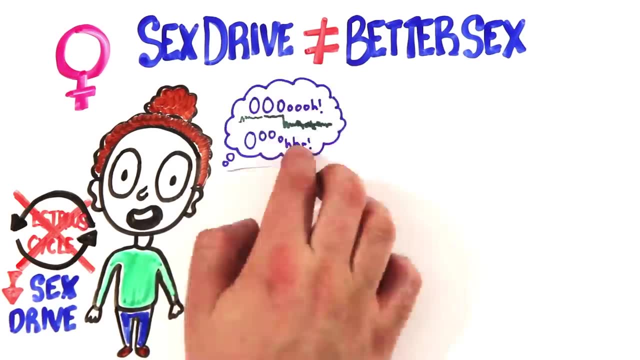 Male mice also become more dominant and are more willing to compete for sex with female mice. But that sex drive may not translate to better sex For female users. steroids can interfere with the estrous cycle and may decrease sexual drive. Masculinization can occur as well, with female users gaining deeper voices. 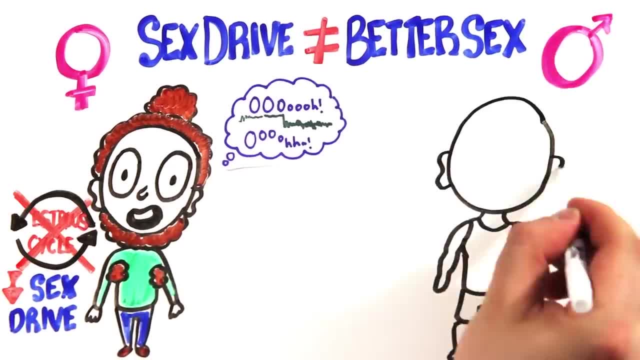 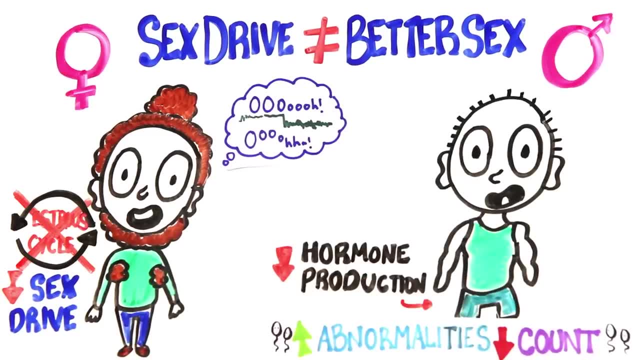 and starting to grow more body and facial hair. Male users may experience sperm cell abnormalities and decreased sperm count. Steroids also decrease natural production of hormones that are necessary for maintaining testicular size, meaning your balls will shrink, And since most steroid users follow a cycle of on and off dosing periods, 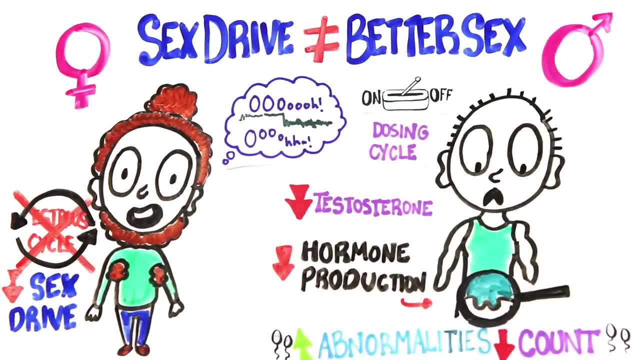 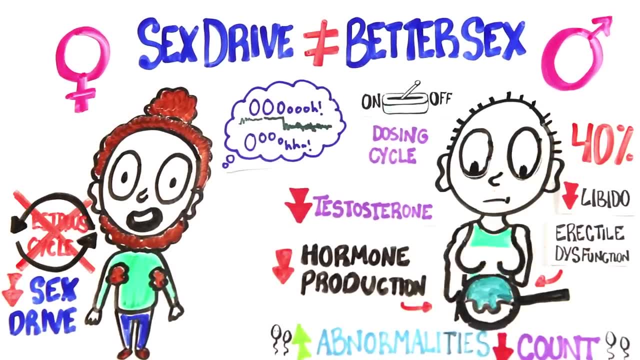 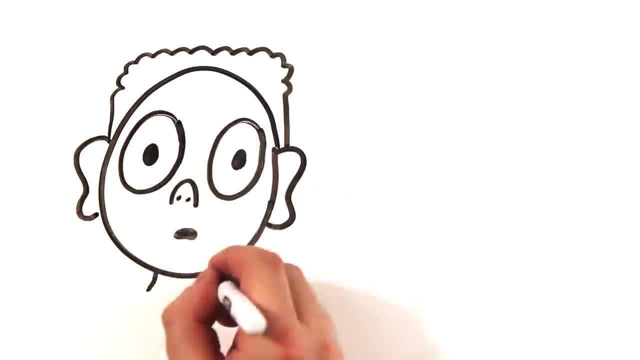 natural levels of testosterone can be quite low at times, causing erectile dysfunction and decreased libido in males. 40% of male users also developed enlarged breast tissue as steroids break down into estradiol, which stimulates the growth of mammary tissue. Finally, steroids can cause a high level of acne in almost half of users.